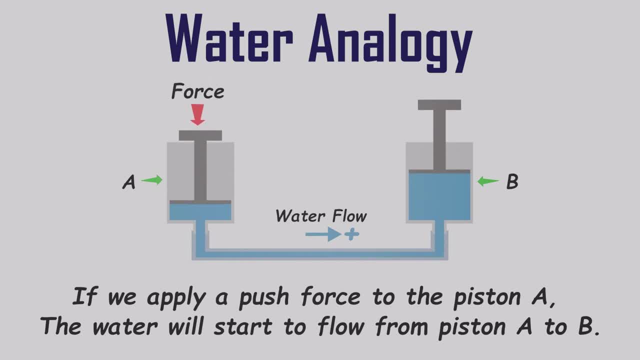 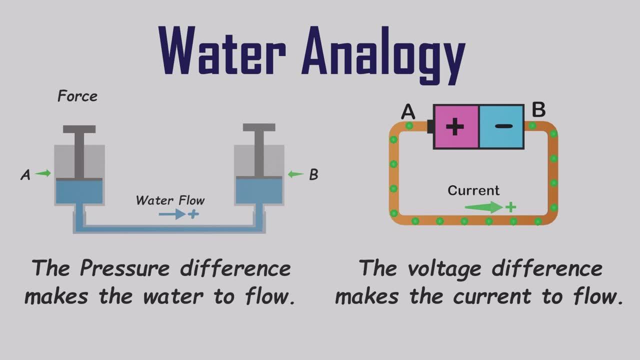 due to increased water pressure. This phenomenon is akin to the flow of electric current in a circuit. When a battery is connected to a circuit, electrons move from the negative terminal to the positive terminal. However, in the context of electricity, we consider current to move from the positive terminal. 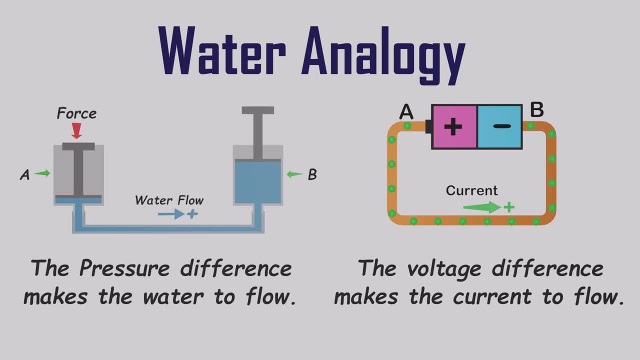 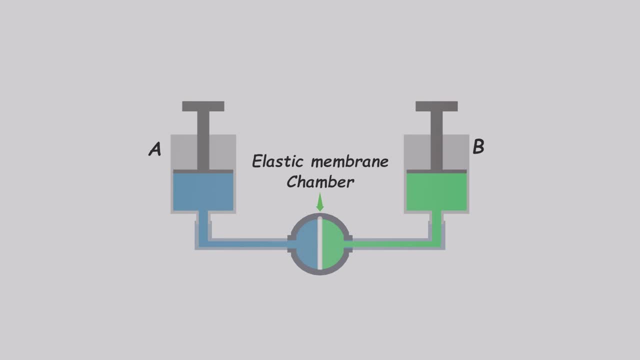 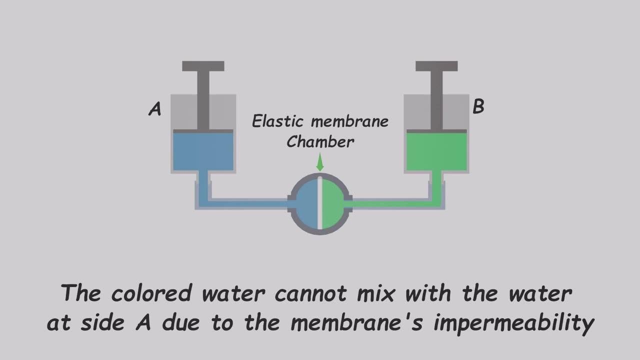 to the low-potential. Here we have an elastic chamber connected to a water pipe acting as a barrier between two sides. Water from side A cannot flow to side B and vice versa. We've dyed the water in side B with green color, but it can't mix with the water in side A due to the membrane's impermeability. 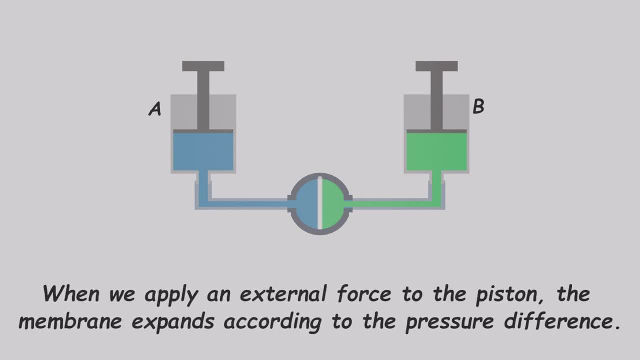 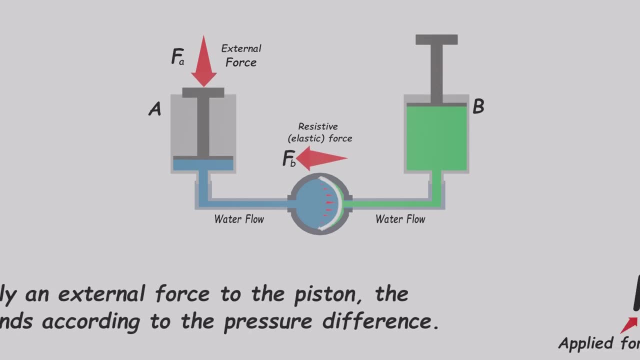 This elastic membrane can stretch to a certain degree, allowing the piston to move, based on the water pressure difference between the two sides. The membrane halts its expansion when the elastic force matches the applied force. Now that we've stored some energy in the membrane, if we disconnect the pistons and connect the two ends of the chamber, 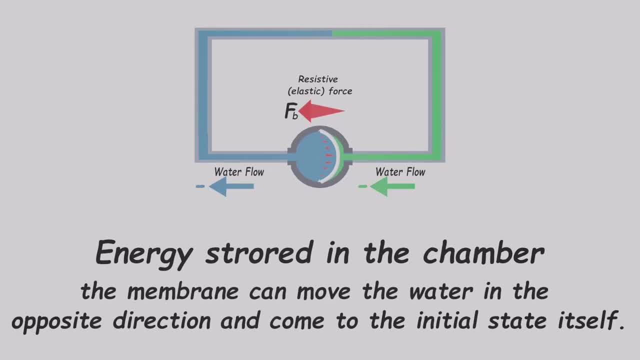 the membrane can move the water in the opposite direction and return to its initial state on its own. Initially we store energy in the device and then we can use the stored energy to do useful work. We can plot the membrane resistance force over time. 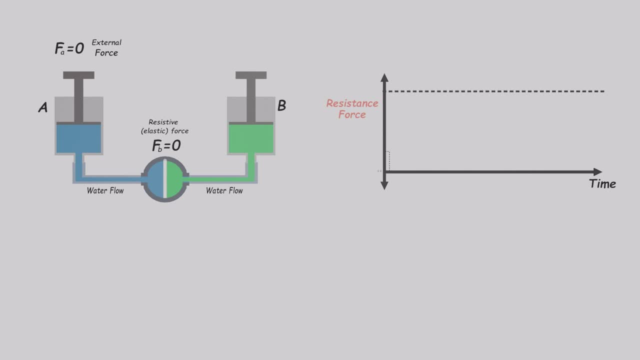 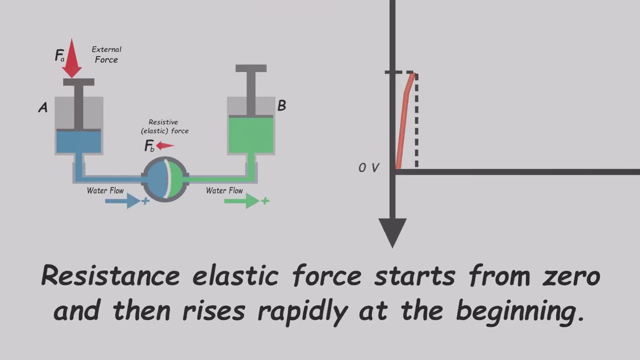 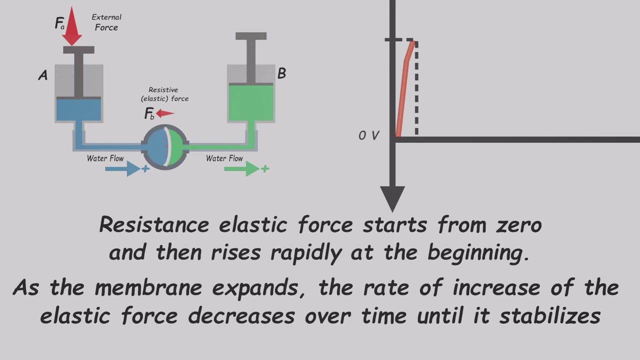 Now let's examine the process in slow motion. Initially, the resistance force is zero. When we apply an external force, the resistance force doesn't increase instantly. It begins from zero and then rises rapidly. However, as the membrane starts to expand, the rate of increase of the elastic force decreases over time. 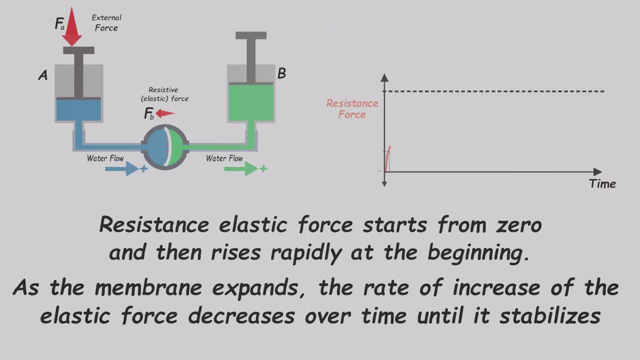 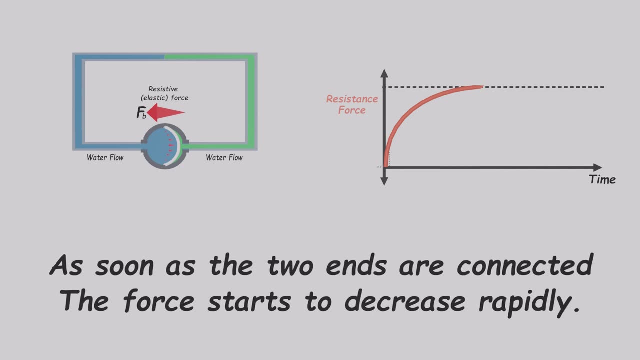 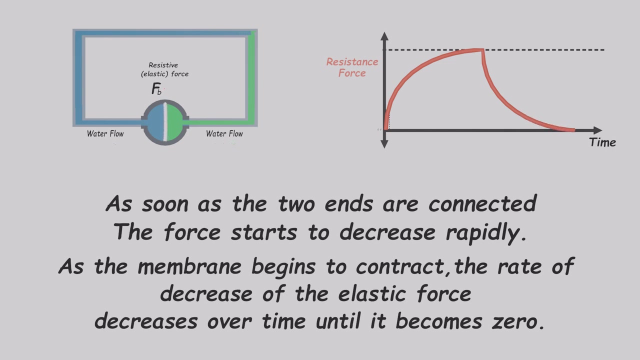 until it reaches zero. This is because the elastic force does not match the applied force. Now let's remove the pistons and connect the two ends. The force begins to decrease rapidly. However, as the membrane starts to contract, the rate of decrease of the elastic force slows down over time until it becomes zero. 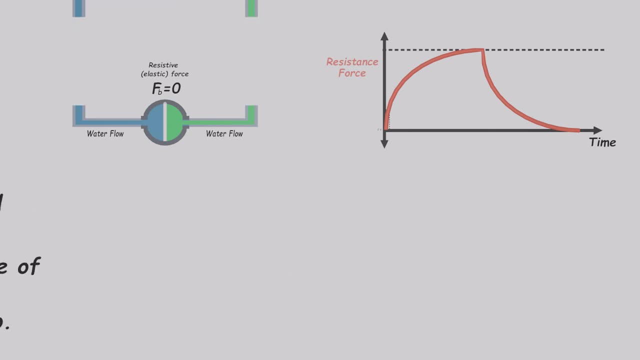 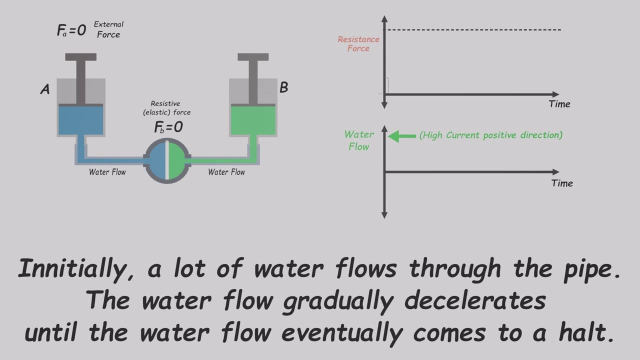 Can you predict what occurs with the water flow during this period? Initially, the membrane is in its resting state, almost as if there is no membrane present at all. Consequently, even a slight force can move a significant amount of water through the pipe. 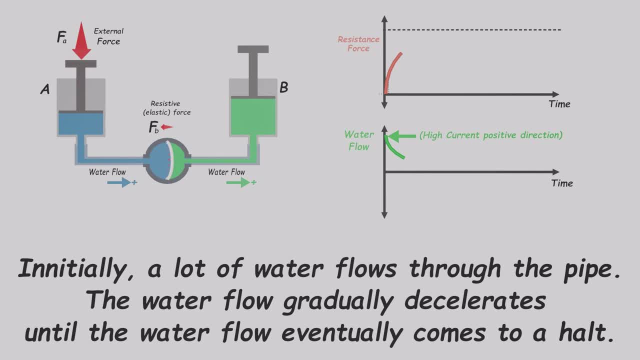 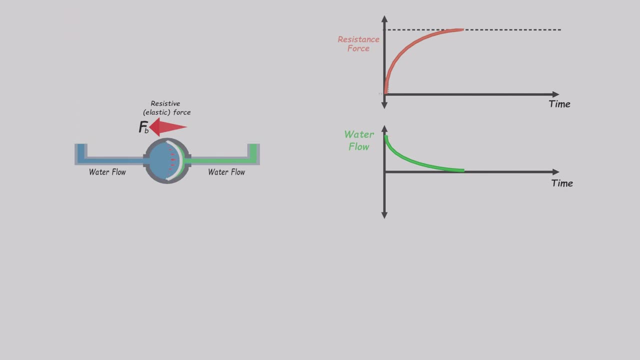 However, as the water begins to move, the membrane expands and starts to exhibit resistance to the water flow, causing it to gradually decelerate. This process continues until the water flow eventually comes to a halt If we remove the pistons and connect the two ends of the chamber. 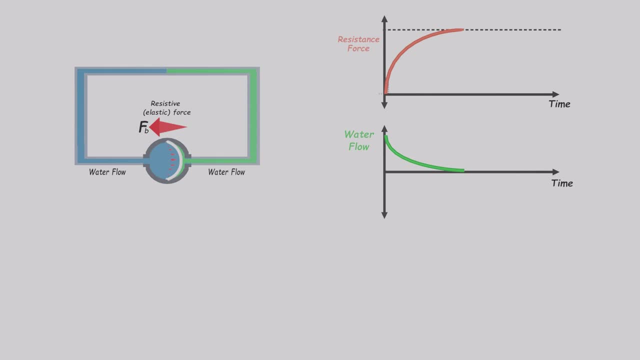 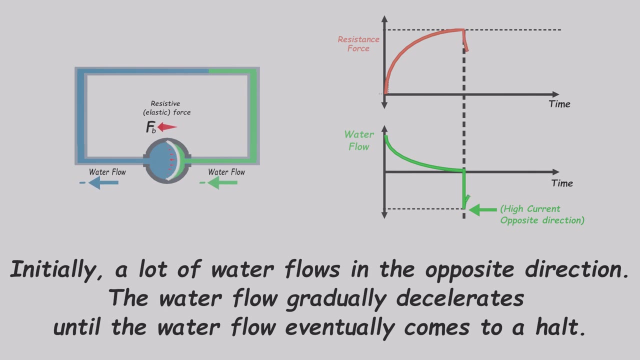 the membrane can move the water in the opposite direction and return to its initial state. Initially, a significant amount of water flows in the opposite direction. However, as the membrane begins to contract, the force decreases, causing the water flow to gradually decelerate. Let's compare these two situations. 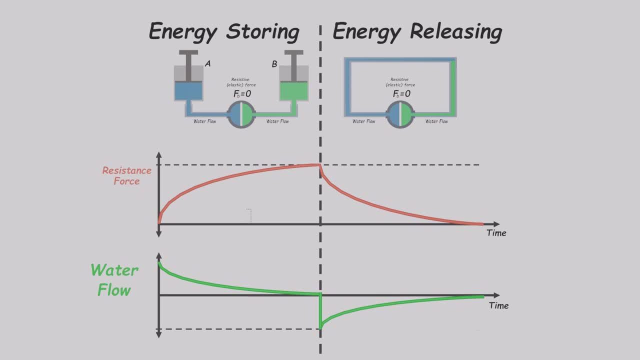 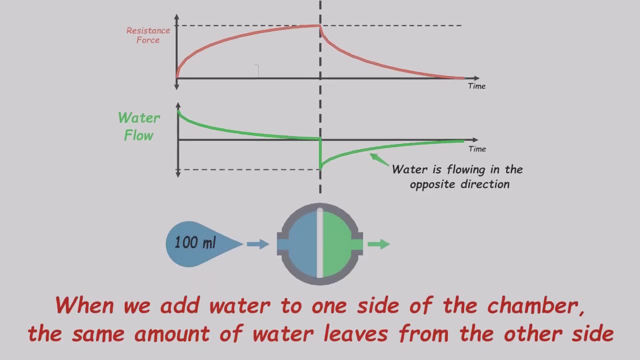 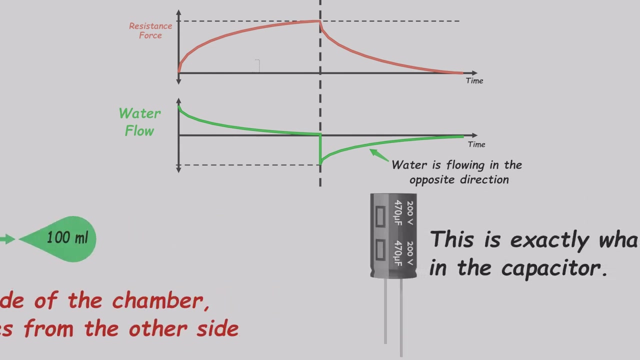 Understanding this water analogy will help you better understand how capacitors work. The negative water flow indicates the water is flowing in the opposite direction. It's important to note that when we add water to one side, the same amount of water leaves from the other side. This is how a capacitor works. 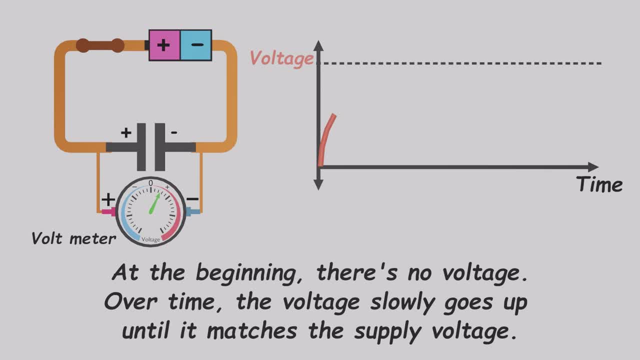 When we connect a capacitor to a battery, here's what happens. At first, the capacitor voltage is zero. Over time, the capacitor voltage is zero. The voltage gradually increases until it matches the supply voltage. If we disconnect the battery and connect the two ends of the capacitor through a resistor, 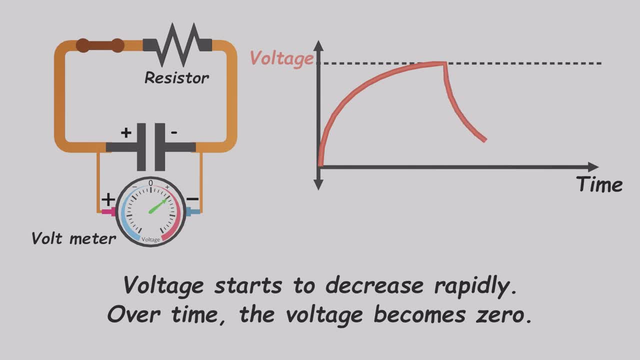 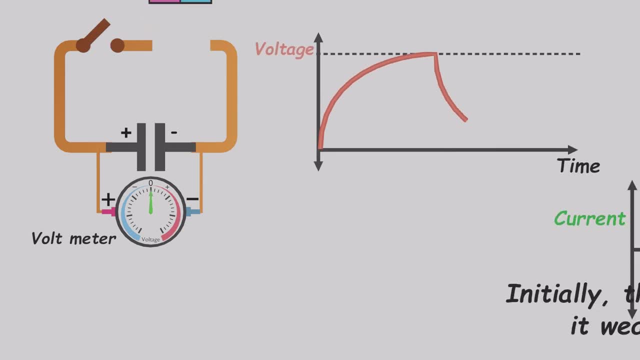 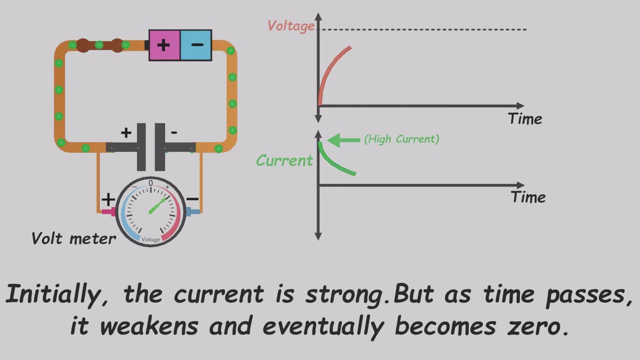 the capacitor voltage starts to decrease quickly until it becomes zero. Now let's consider the current. In the beginning, the current is high. However, as time progresses it diminishes and eventually reaches zero If we disconnect the battery and connect the two ends of the capacitor through a resistor. 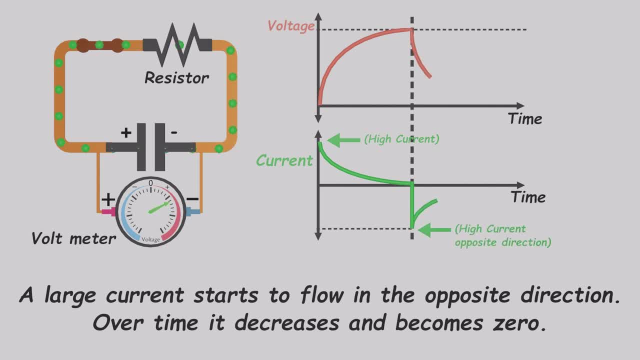 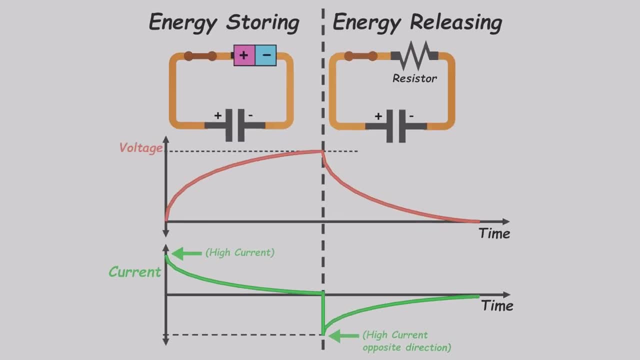 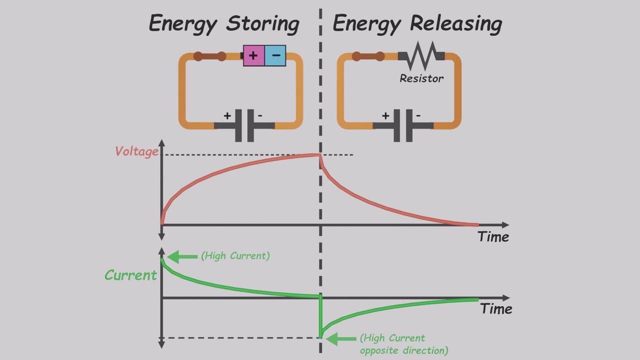 a significant current starts flowing in the opposite direction. Over time, this current diminishes and becomes zero. Here, voltage behaves similarly to the membrane force, as seen in the earlier example. Similarly, current behaves like the water flow in the analogy. Let's explore this further. 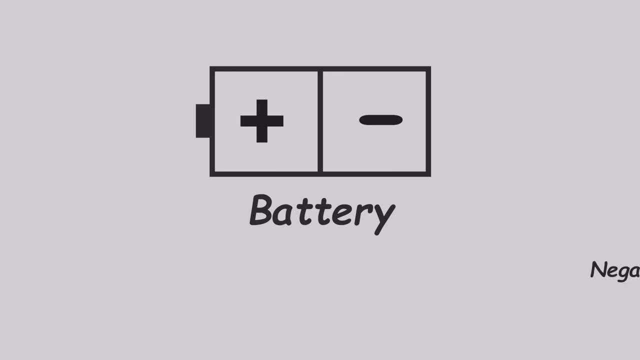 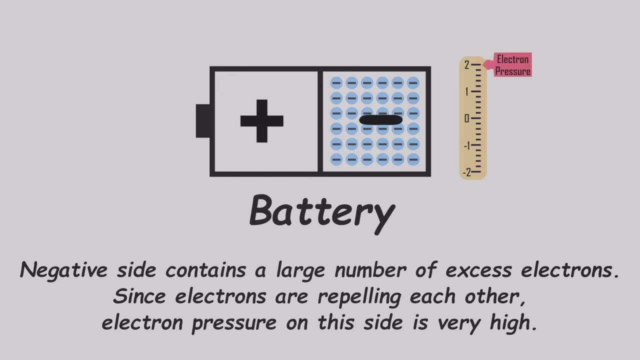 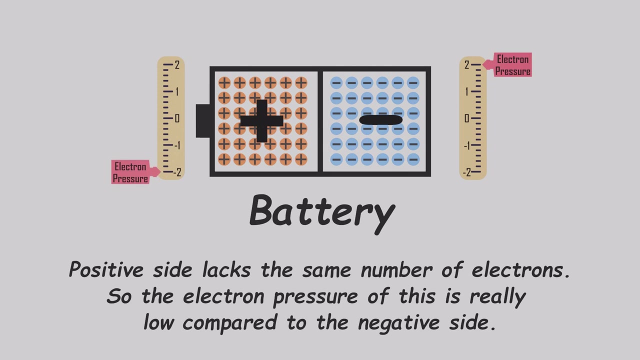 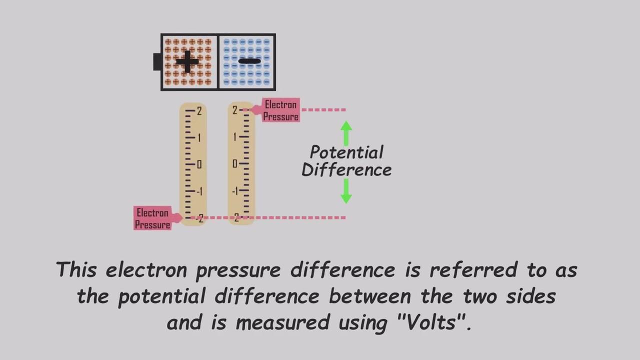 Imagine a battery with positive and negative sides. The negative side holds a surplus of electrons, leading to high electron pressure. In contrast, the positive side lacks the same number of electrons, creating a lower electron pressure compared to the negative side. This difference in electron pressure is known as the potential difference, measured in volts. 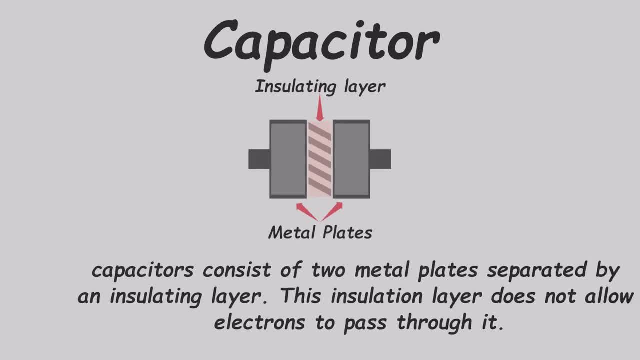 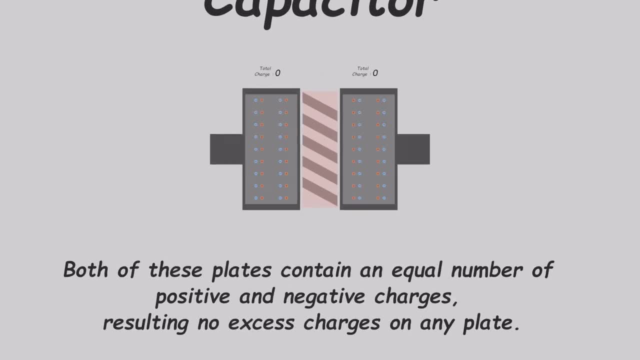 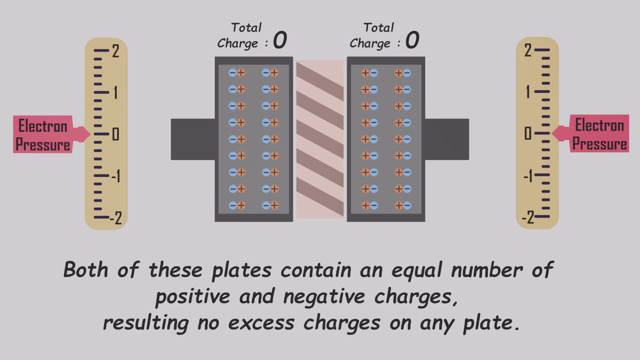 Let's turn our attention to the capacitor. It consists of two metal plates separated by an insulating layer that prevents electron flow. Initially, both plates have an equal number of positive and negative charges, resulting in a neutral state with zero total charge. Therefore, the electron pressure on the plates can be seen as zero. 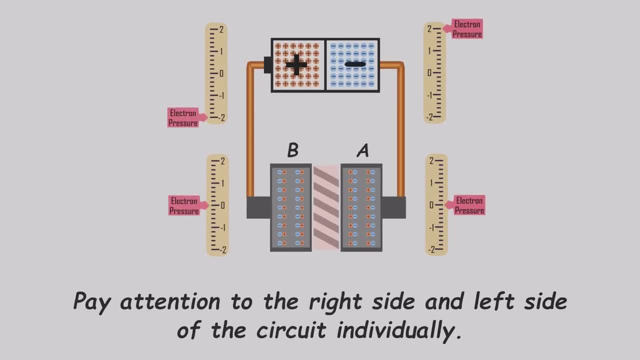 Let's connect the capacitor to a battery. Focus on the right side of the circuit Electrons from the negative side. see that the capacitor's plate A has less than one electron per second electron pressure compared to the negative side of the battery. Thus they try to move. 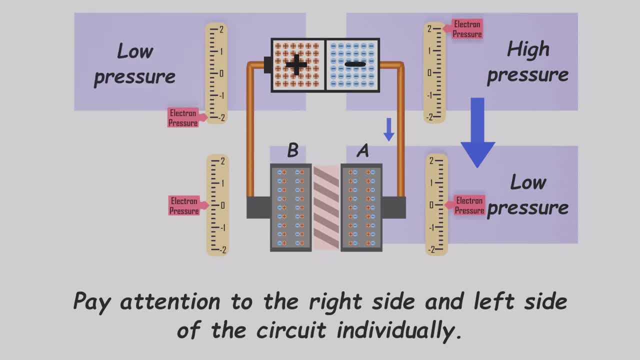 towards plate A. Similarly, on the left side, electrons in plate B of the capacitor move towards the positive side of the battery, attracted by the lower electron pressure. Remember, the electrons can't cross the insulating layer, so as one plate gains an electron. 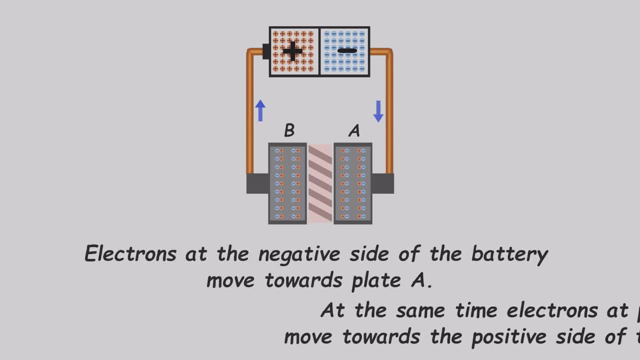 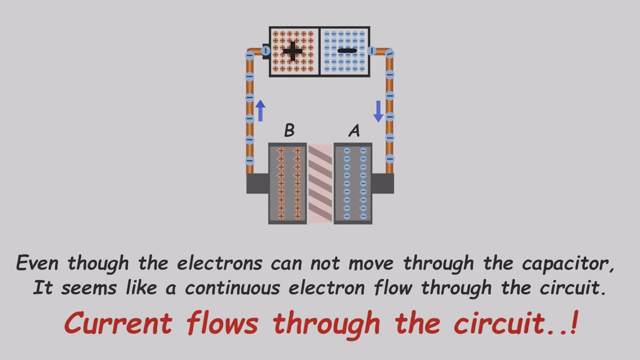 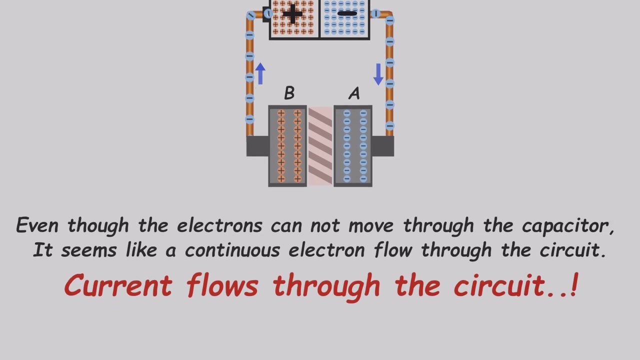 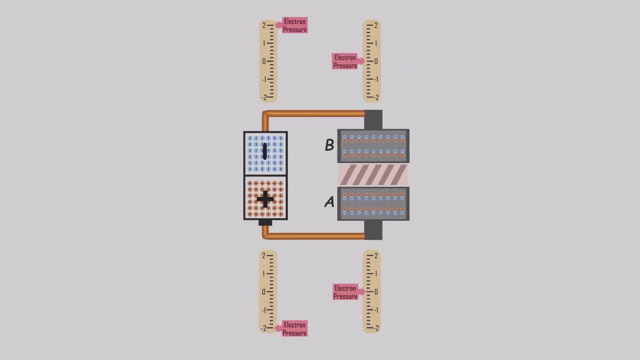 the other releases one. This creates the effect of a continuous electron flow, resembling a current through the circuit. Let's examine the changes in electron pressure. I'll represent the electron pressure of each end using scales. Initially, there's a significant difference in electron pressure. 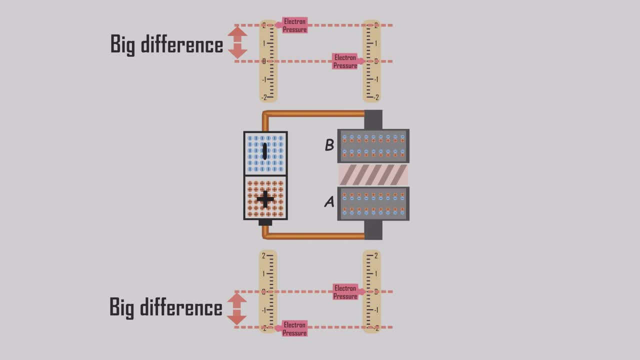 between the battery and the connected plates. This prompts electrons to move towards the negative side of the battery. attracted by the negative side of the battery, This causes electrons to move towards regions with lower pressure. Consequently, the electron pressure increases on one plate and decreases on the. 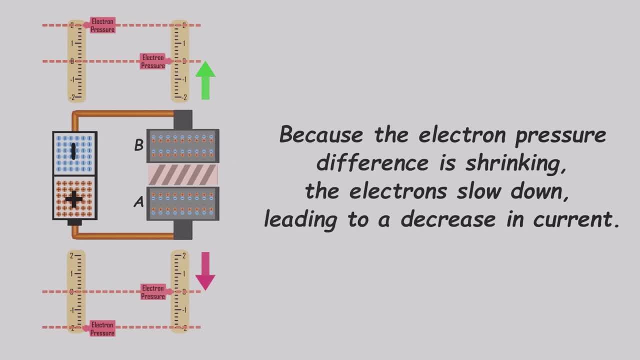 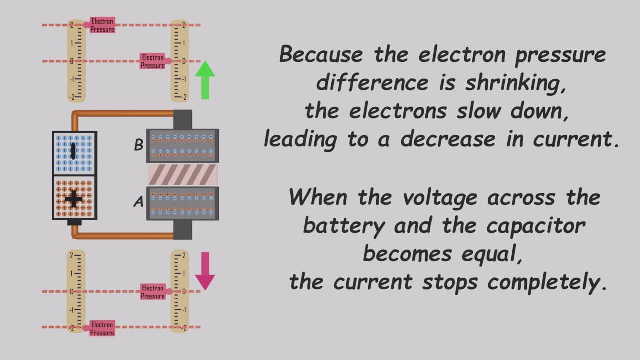 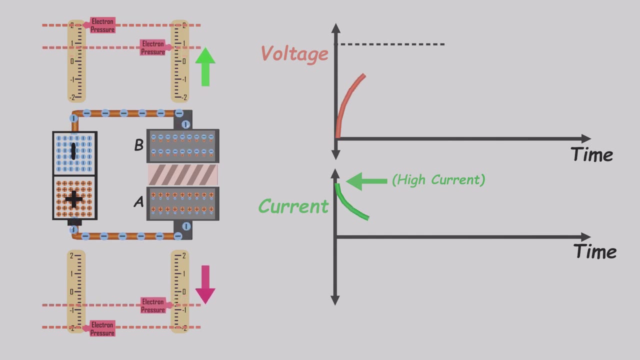 other. As the electron pressure difference diminishes, the electron speed slows down, causing a decrease in current. Eventually, when the voltage across the battery and the capacitor becomes equal, the current stops entirely. This clarifies why the voltage difference between the two plates begins at zero and gradually increases. It also explains why 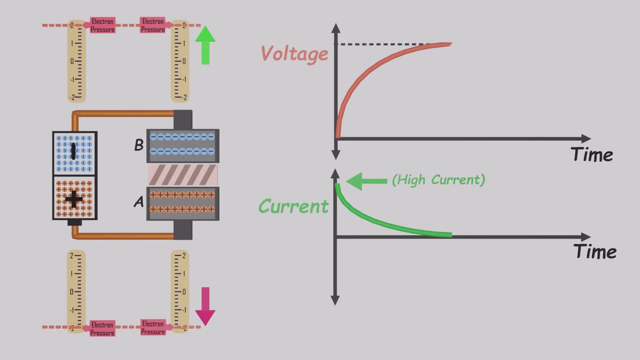 the current decreases over time. and the current decreases over time. It's important to note that as electrons move, the battery's voltage undergoes a slight change, but this alteration is minimal and can be disregarded compared to the capacitor's voltage change. Now let's remove the battery and connect the two ends of the capacitor through a resistor. 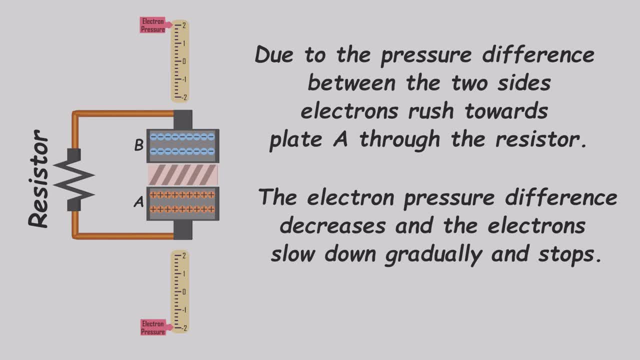 Initially, there is a significant electron pressure in plate B and a very low electron pressure in plate A. Consequently, electrons rush towards plate A through the resistor, resulting in a high current, but in the opposite direction. Over time, the electron pressure difference decreases, causing the electrons to slow down gradually. When the pressure 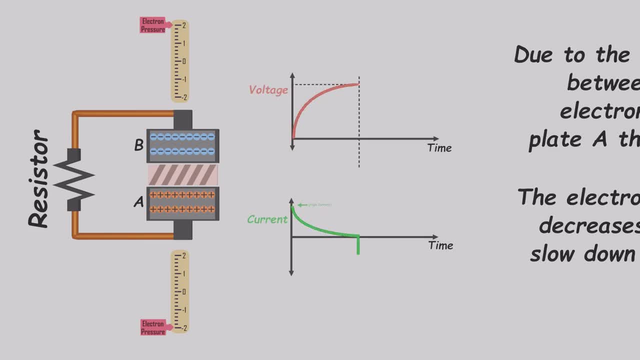 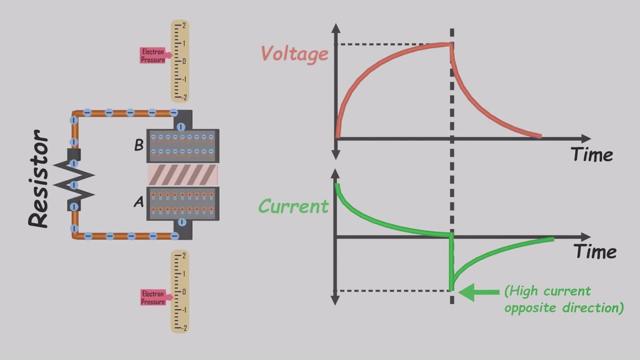 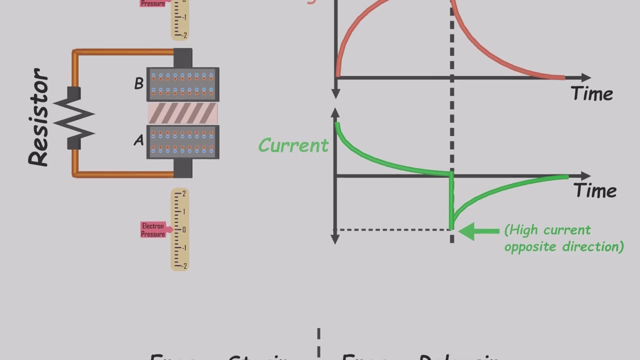 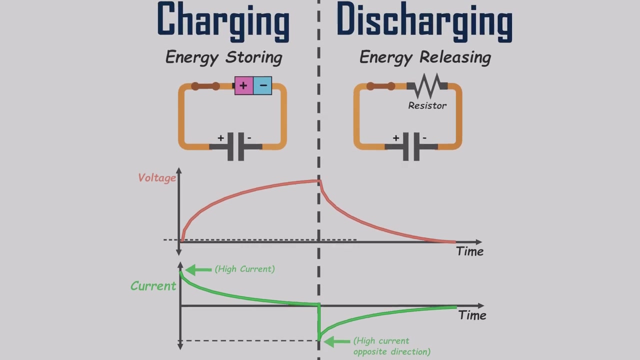 difference reaches zero, the current stops. Now that we have a basic understanding of what's happening with band A, we can think of capacitors. we can explore their behavior further. When we store energy in a capacitor, it is known as capacitor charging. 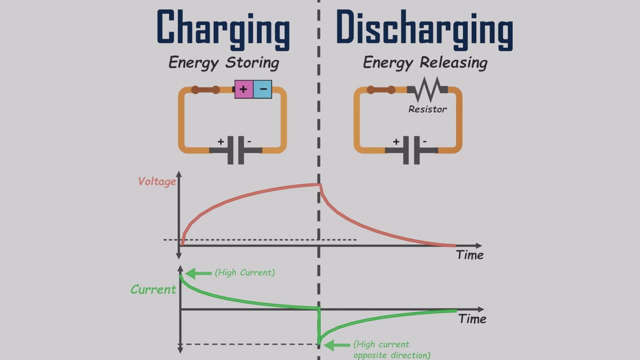 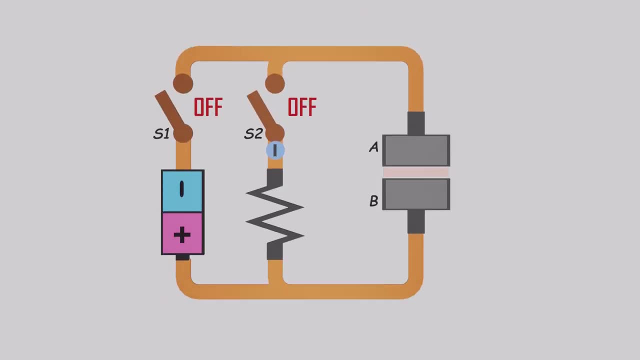 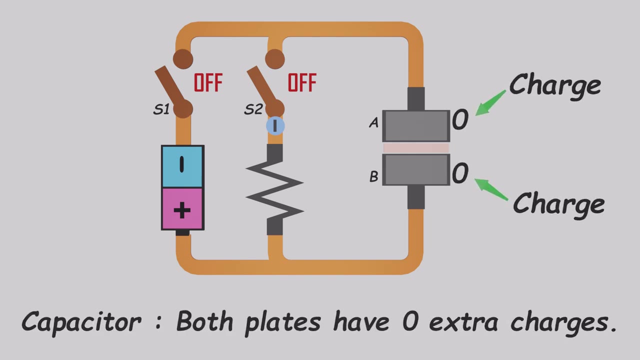 Conversely, when we use the stored energy, it is termed as capacitor discharging. Let's continue our exploration. We've modified our circuit to observe capacitor charging and discharging. Initially, both plates are charged neutral, resulting in zero capacitor voltage If we turn on switch S1,. 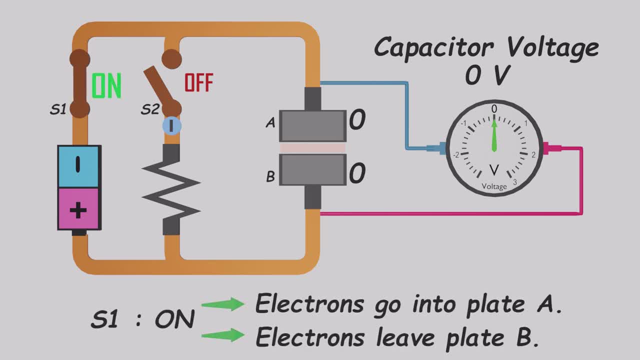 current will flow and the capacitor will start to charge. Let's consider what happens in detail. When one electron moves to plate A, its charge becomes minus one, And another electron leaving plate B brings its total charge to plus one. This slight difference in charge. 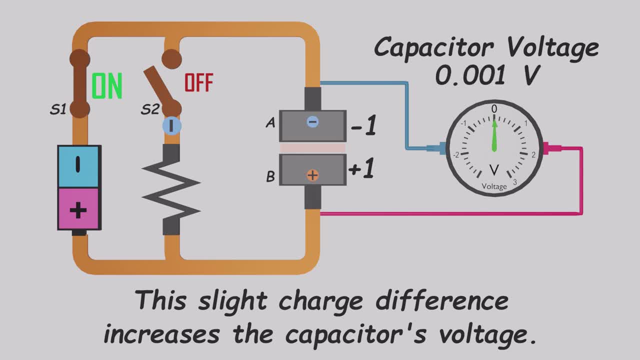 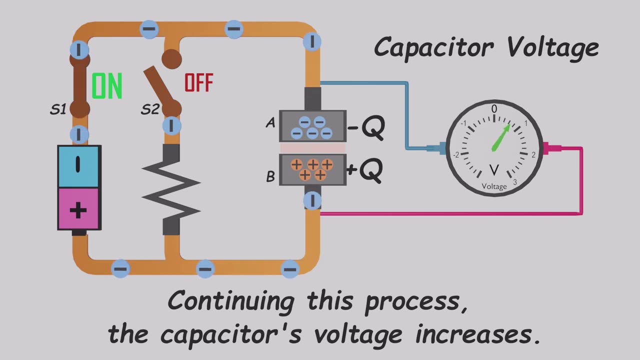 causes an increase in the capacitor's voltage. Continuing this study, we can see that the capacitor's voltage increases. This process alters the total charge on both plates, consequently increasing the capacitor's voltage. The coulomb is the unit of electric charge in the international. 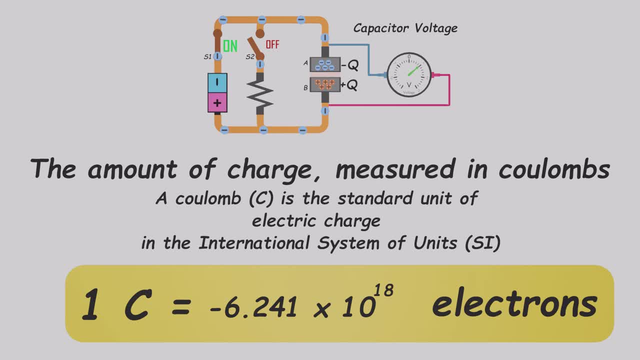 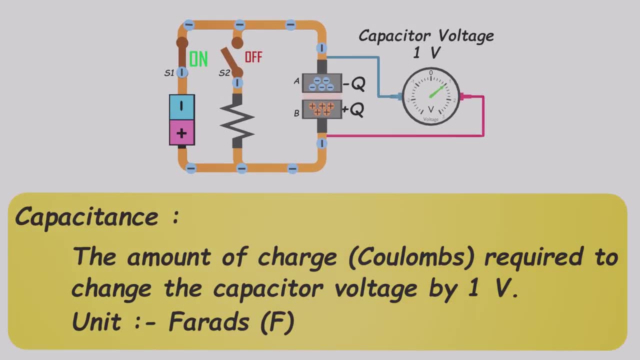 system of units. One coulomb is equal to approximately six quintillion positive or negative charges. The capacitance of a capacitor is the amount of charge measured in coulombs needed to change the voltage across the capacitor by one volt. Capacitance is measured in units called farads. Let's assume 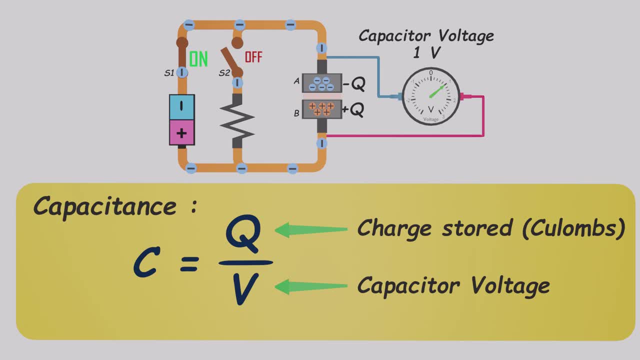 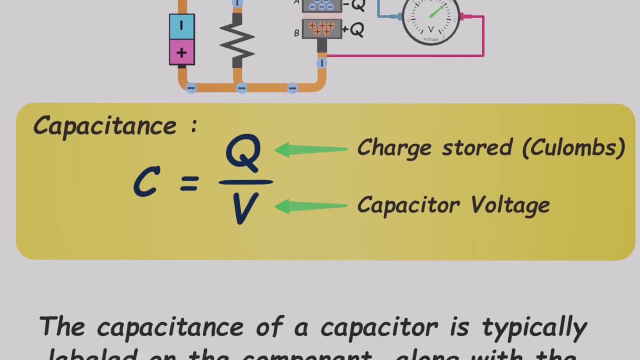 this capacitor needs Q coulombs of charge for each plate to change its voltage by V volts. We can find the capacitance of this capacitor by dividing Q by V. The capacitance of a capacitor is typically labeled on the component, along with the voltage rating and other details. 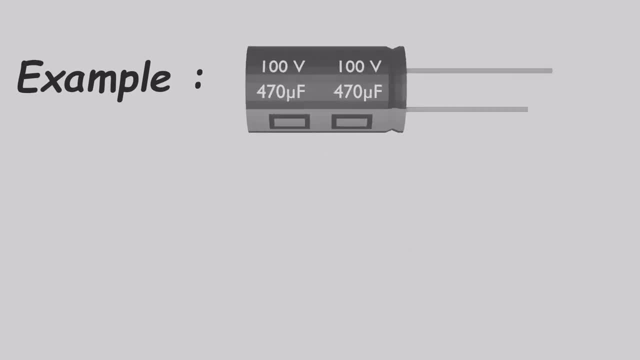 For instance, a capacitor might be marked as 100 volts and 470 microfarads. This means the capacitor has a capacitance of 470 microfarads. In simple terms, it requires 470 microcoulombs of charge to change its voltage by one volt. 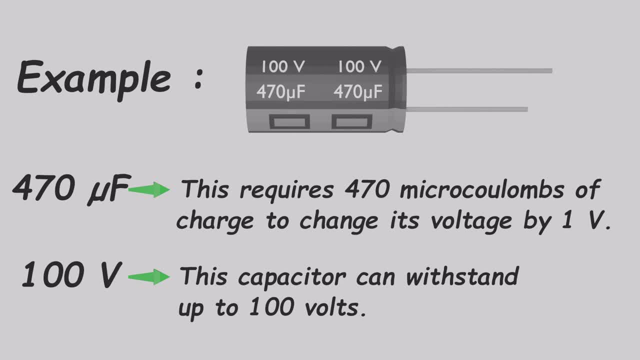 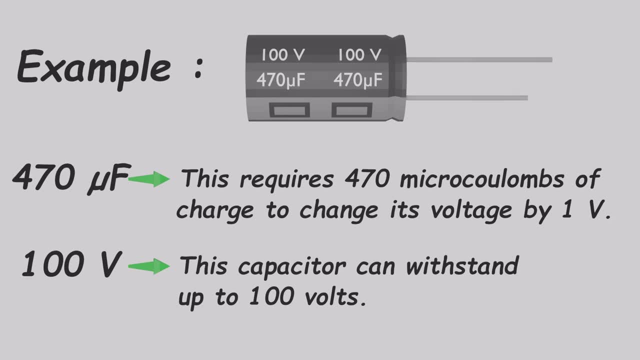 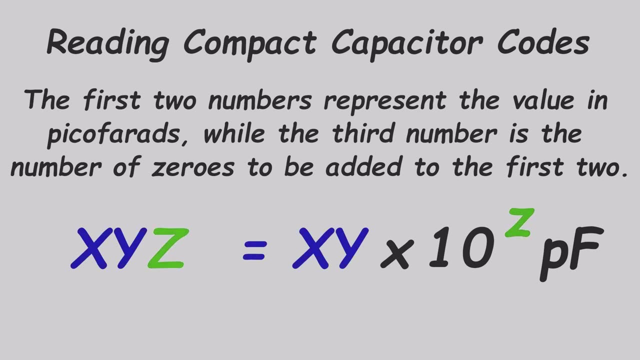 The voltage rating indicates the maximum voltage the capacitor can handle without getting damaged. In this case, the capacitor can withstand up to 100 volts. Some tiny ceramic capacitors have two to three digits code printed on them. The first two numbers describe the value of the capacitor and the third number is the number of zeros. 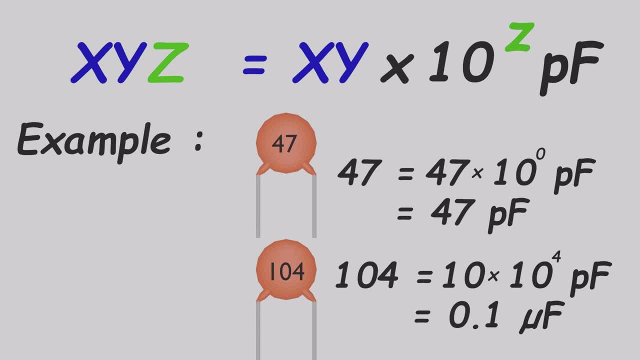 in the multiplier. When the first two numbers are multiplied with the multiplier, the resulting value is the value of the capacitor in picofarads. If there are only two numbers, it means there is no multiplier. You can read the value of the first two numbers in picofarads: 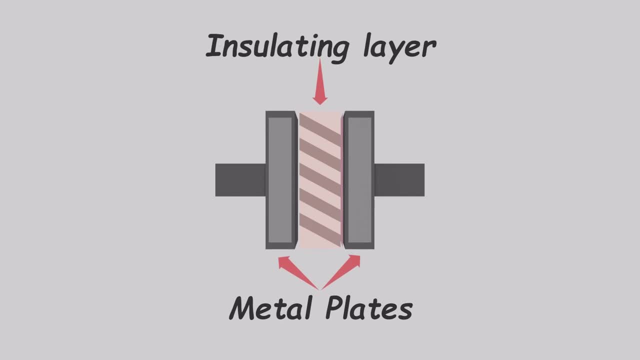 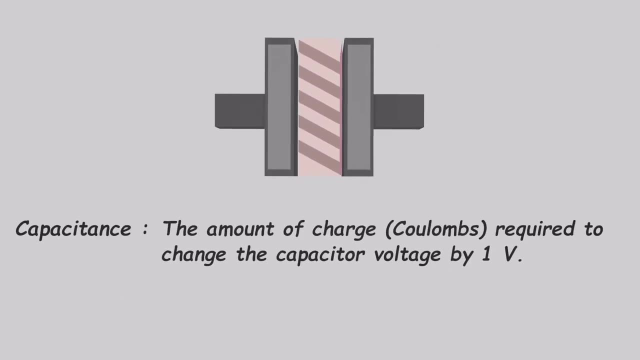 Let's revisit the construction of the capacitor. It consists of two metal plates separated by an insulating material layer. The capacitor's capacitance, indicating the charge it needs to change its voltage by one volt, depends on three main factors: The surface area of the conductors. the distance between the conductors. 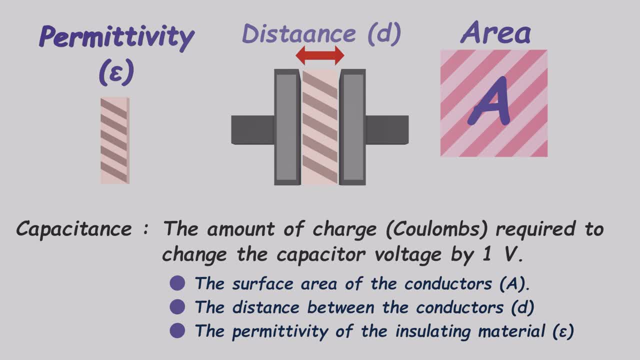 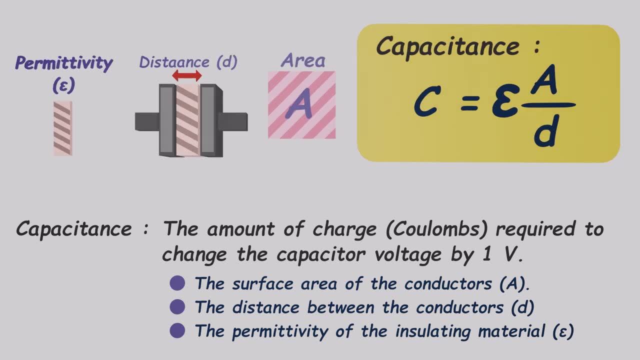 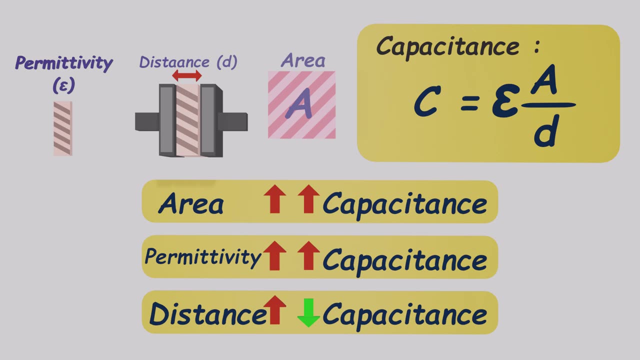 and the unique permittivity of the insulating material, which depends on the material. We can calculate the capacitance using the equation: Capacitance increases with the surface area of the conductors and the permittivity of the insulating material, while it decreases with the distance. 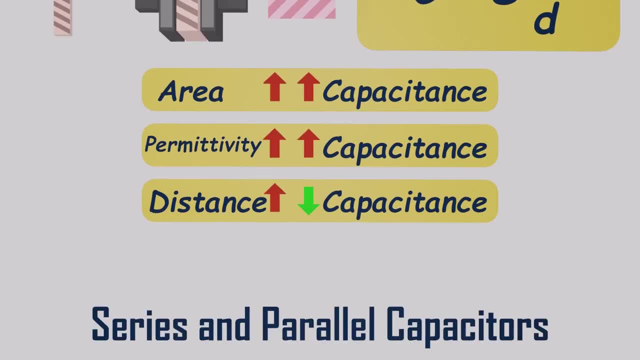 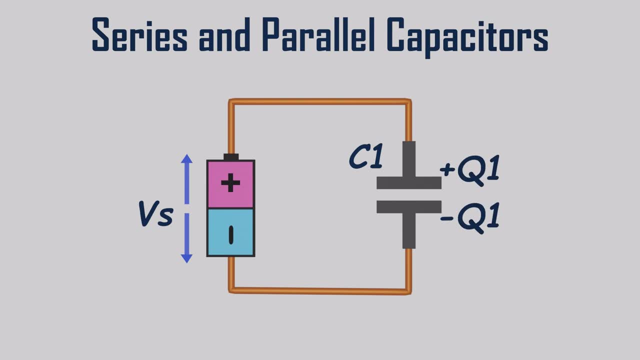 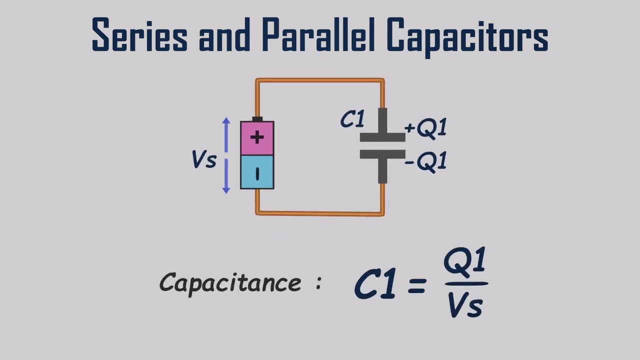 between the conductors. We have a circuit like this. Let's assume this capacitor needs Q1- amount of charge to reach the battery voltage Vs. As we discussed earlier, the capacitance of the circuit is given by the formula C1, equal to Q1 divided by Vs. Now we need to add another capacitor. 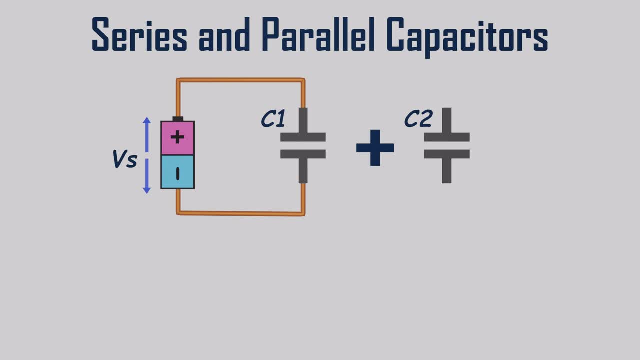 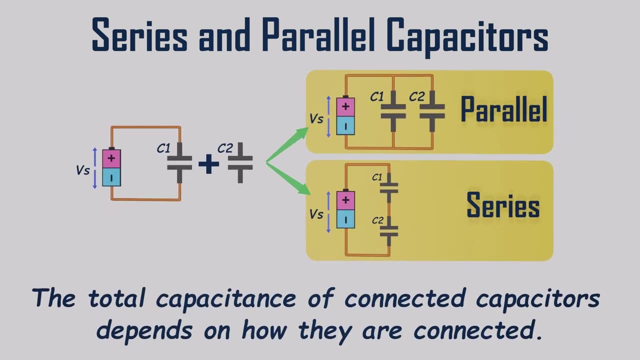 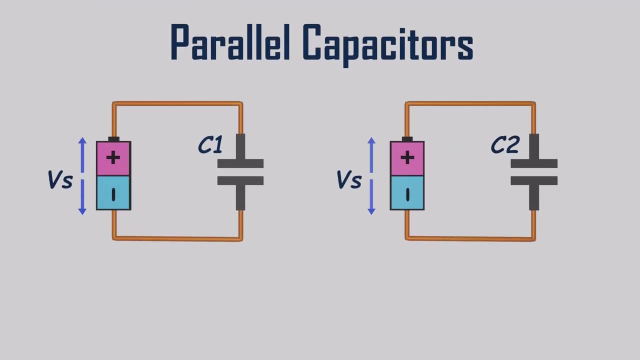 to this circuit. How can we do that? We have two options: Parallel or series connection. The total capacitance of the capacitors changes depending on the selected connection method. Let's consider the parallel arrangement. Imagine both capacitors are connected to separate. batteries like this Suppose to increase the voltage up to the battery. 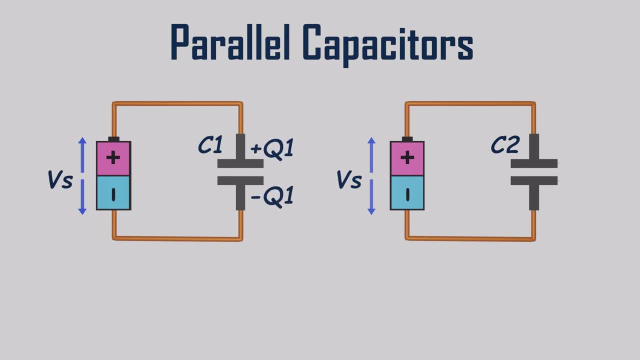 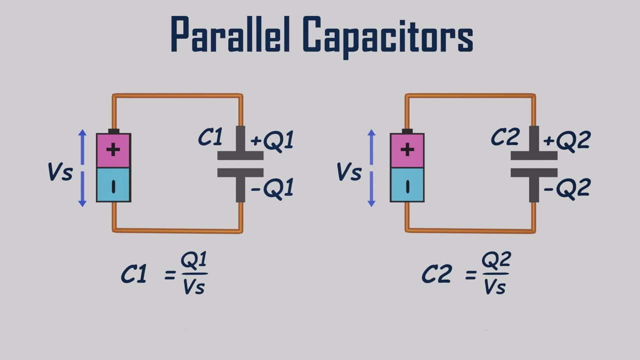 voltage. C1 needs Q1 amount of charge and C2 needs Q2 amount of charge. We can express Q1 and Q2 using the voltage and capacitance of each capacitor. Let's rearrange these equations to make Q the subject Now. 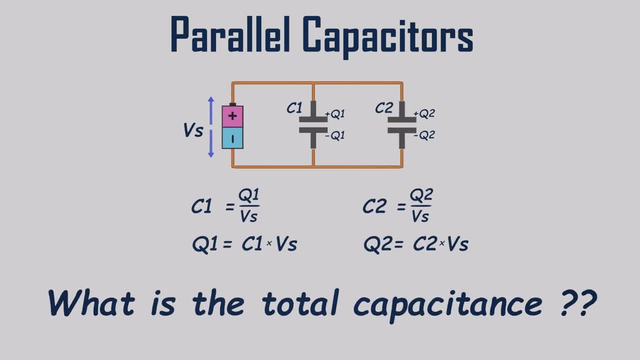 instead of two batteries if we connect both capacitors to one battery like this, C1 still needs Q1 and C2 needs Q2 to reach the supply voltage level. To determine the total capacitance of this circuit, consider a single equivalent capacitor. 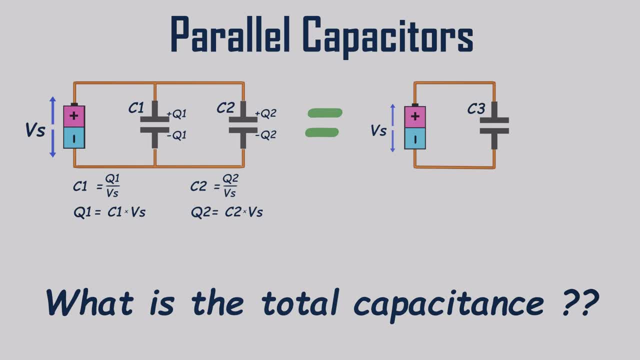 that replicates the combined effect of C1 and C2.. This equivalent capacitor will have a capacitance value that represents the total capacitance of the circuit. This capacitor, C3, needs Q1 plus Q2 amount of charge to reach the supply voltage. So we can write the capacitance of C3 as Q1 plus. 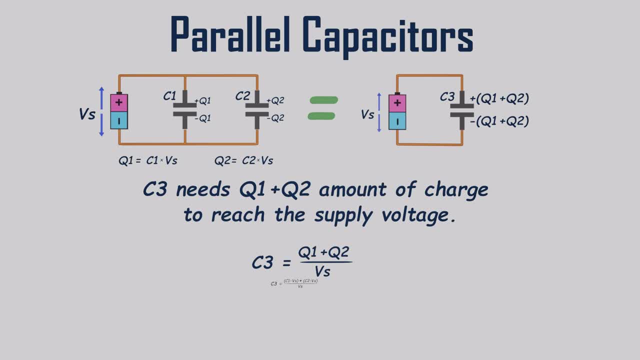 Q2 divided by Vs. Here we can replace the Q1 and Q2 from the C1, C2 and Vs. We can simplify this expression by canceling common factors, resulting in a relationship like this: In conclusion, when capacitors are connected in parallel. 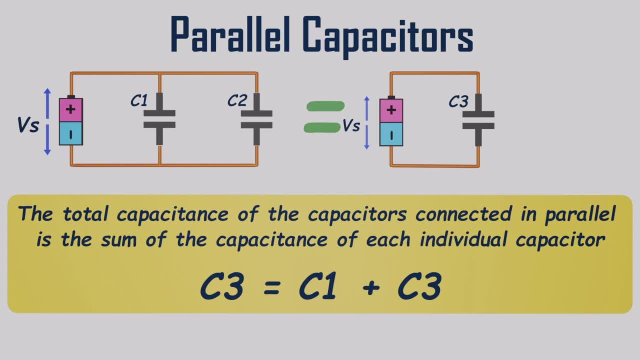 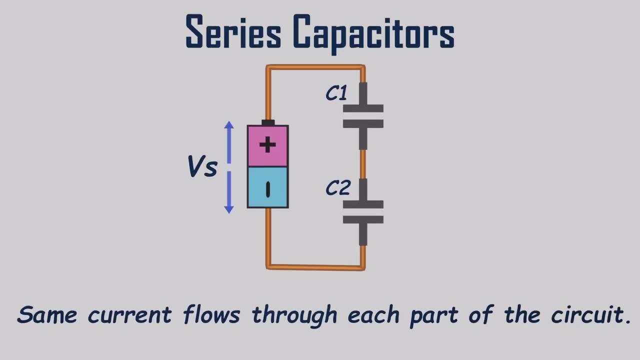 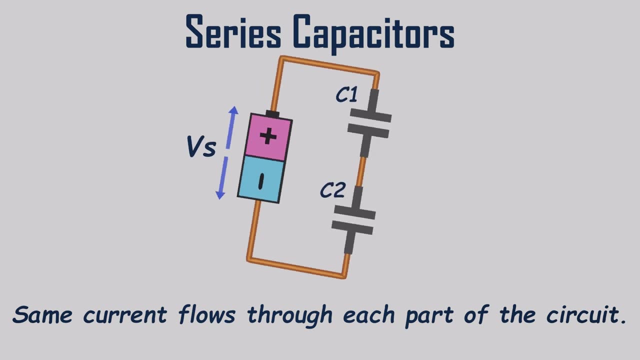 the total capacitance of the system is just the sum of the capacitance of each individual capacitor In a series capacitive circuit. the same displacement current flows through each part of the circuit. Let's examine this more closely. For clarity, let's name the plates as P, Q, R and S. 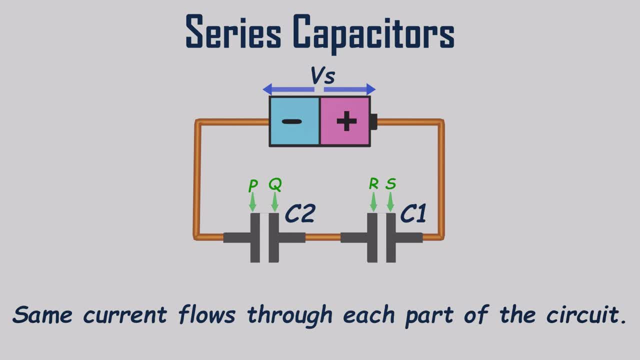 If one electron moves from the negative side to plate P of C1, one electron has to leave plate Q to plate R of C2.. This process continues where, to accumulate one electron on plate R, plate S has to release one of its electrons. 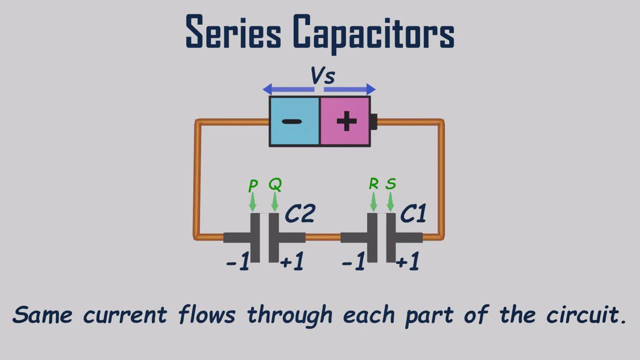 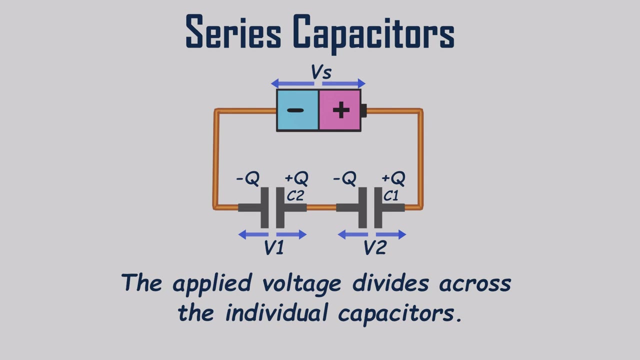 These electron movements occur simultaneously, Hence each plate always holds the same amount of charge and the applied voltage divides across the individual capacitors. Now we can proceed to calculate the capacitance of each of these capacitors. Let's rearrange these equations to isolate voltage as the subject. 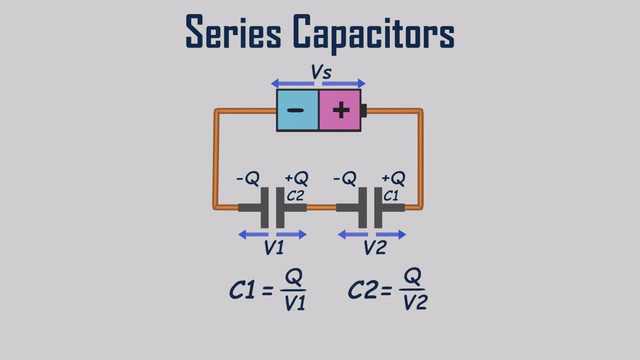 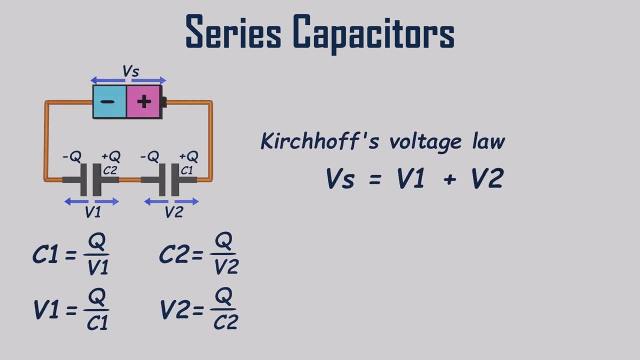 According to Kirchhoff's voltage law, the sum of the capacitor voltages must equal the source voltage By replacing V1 and V2 with the capacitance of each capacitor. the sum of the capacitor voltages must equal the source voltage By multiplying V1 and V2 with the capacitance of each capacitor.